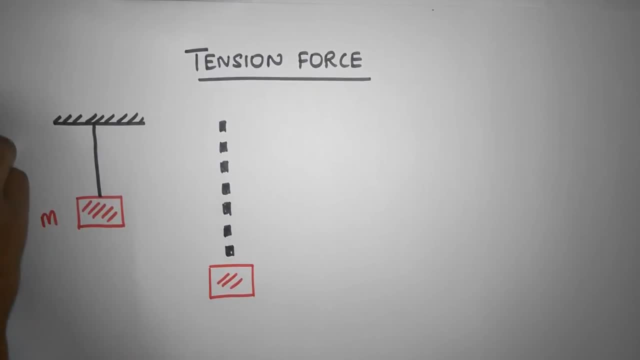 Like. so Now notice that there is a gravitational force acting on this block. Let's put mg using blue. So there is mg. Now what's going to happen is because there's an intermolecular force between the string and this particular block. this string will put a force back on the block, upwards, and that's going to be the tension force, And I'm going to use green in this example to depict the tension force. 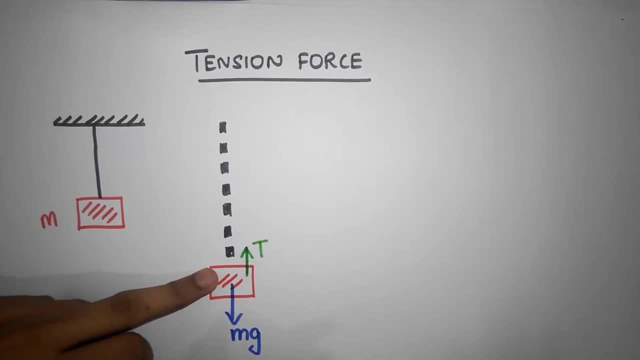 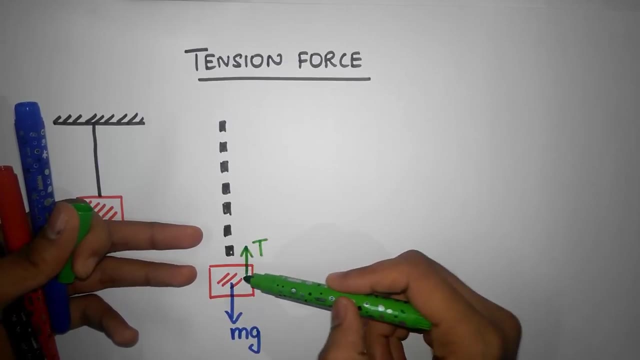 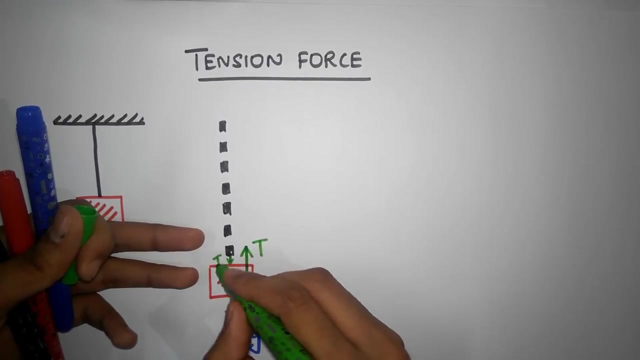 This way. But remember Newton's Third Law: If the string puts a tension force on the block, the block puts a tension force back on the string. So the block is pulling this chunk of the string down with the tension force T. I hope you don't get confused These two. 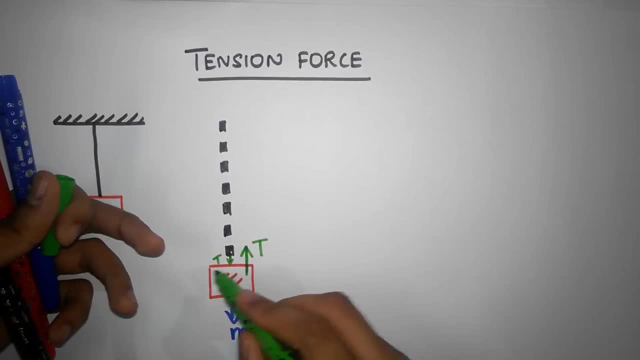 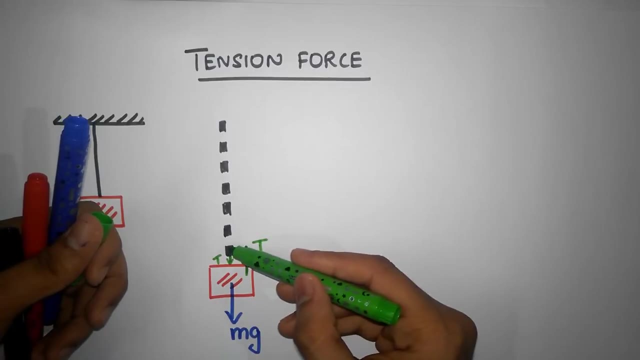 tension forces don't cancel each other out. if you are worrying about the block, then only the tension force. this tension force and mg are acting. If you consider this part of the string, then there's another tension force down acting, that's T. But then what's going to happen is this string is going to pull this guy up. 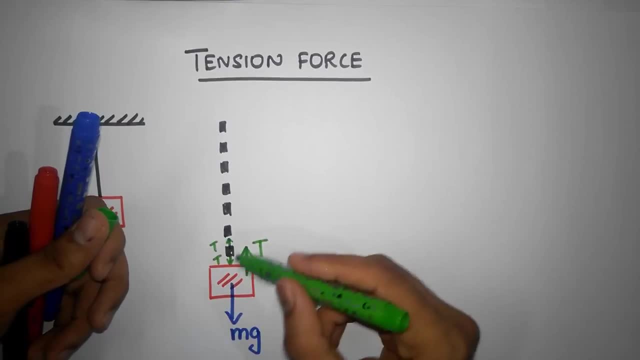 with the force T, So the total force on the string becomes zero, because there are two tension forces acting on the opposite direction. And I can do the same thing on this guy. Since this guy is pulling this fellow up, this fellow will pull this guy down. so there's a tension. 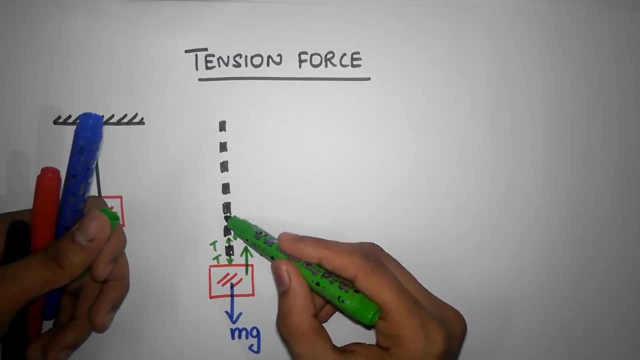 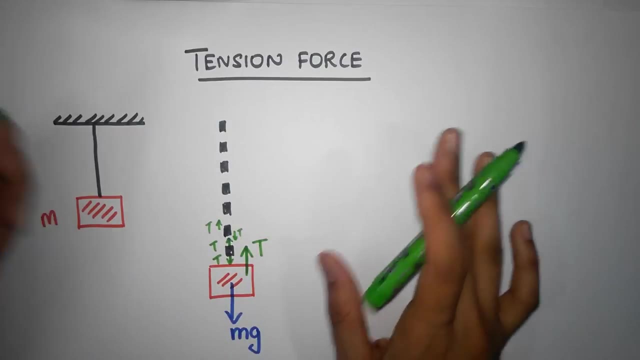 force T acting down on this fellow, And similarly, this guy will pull him up with the tension force T And notice that everywhere the tension is going to remain exactly the same T. That's the whole idea behind the tension force. Notice that the tension force is a pulling force. 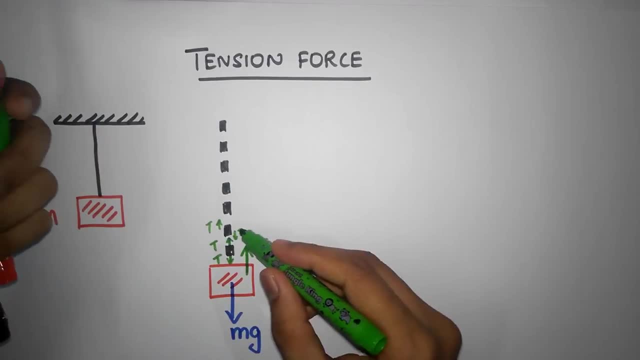 Each bit of the string is being pulled with some force T, And we can now evaluate how much that force is supposed to be. Let's put: F equals ma for this block. So I'm going to call this as the y direction. I'm going to say sigma F in the y should be equal to mass. 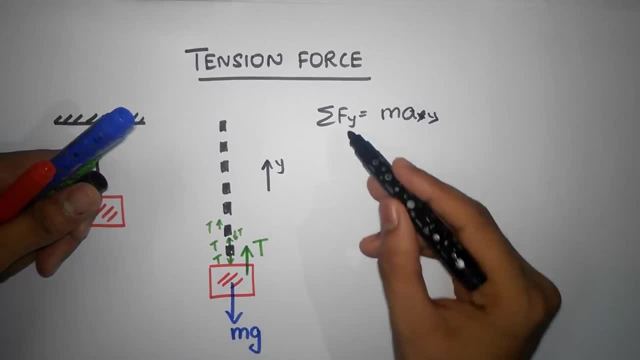 times the acceleration in the y direction. And I'm going to say sigma F in the y direction, I'm going to say sigma F in the y direction, I'm going to say sigma F in the y direction. There are two forces acting in the y direction. There's a tension force acting upwards and 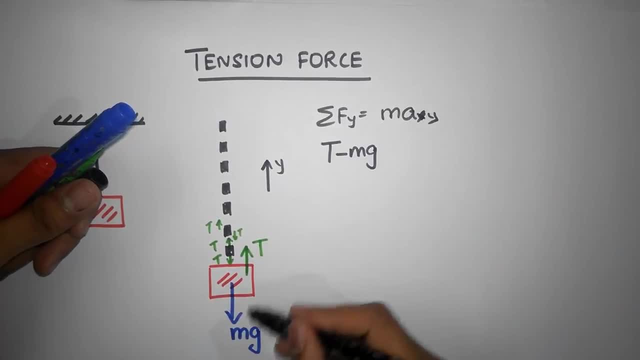 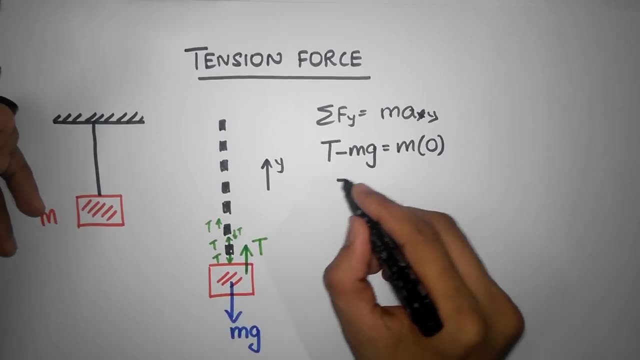 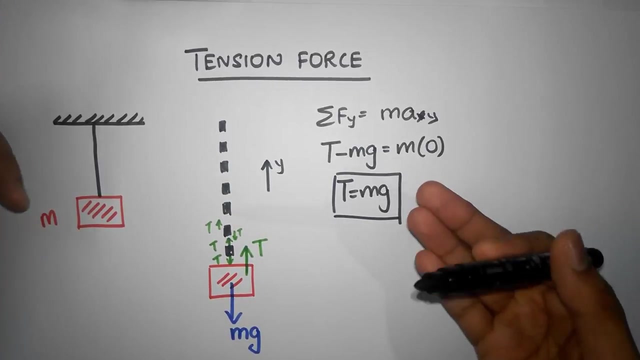 there's an mg acting downwards on this fellow, So there's a minus sign because it's downwards. It should be equal to mass times acceleration, but there is no acceleration, As I told you, it's just standing still. So tension must be equal to mg. This is not always the case. 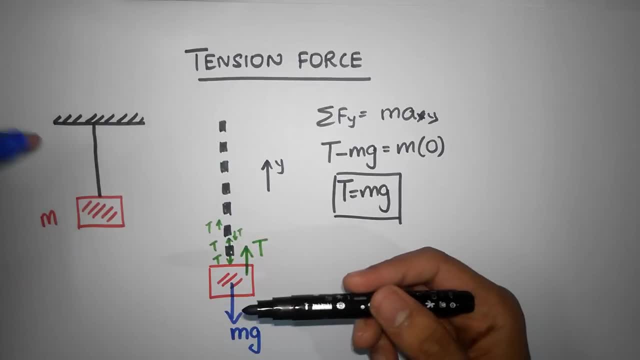 It's the case in this particular example. Okay, And we're going to always assume that most of the time. we're going to assume that the strings are massless. Okay, And if the strings are massless, the tension force everywhere in the string must be exactly the same It. 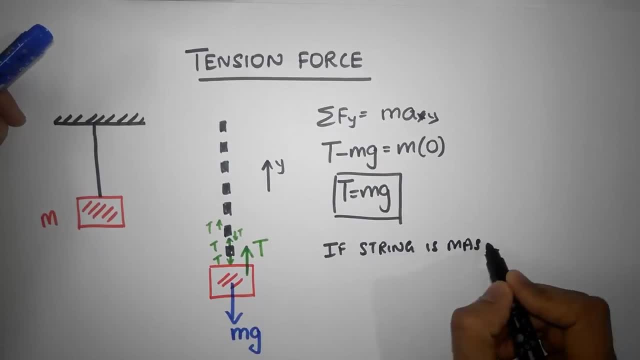 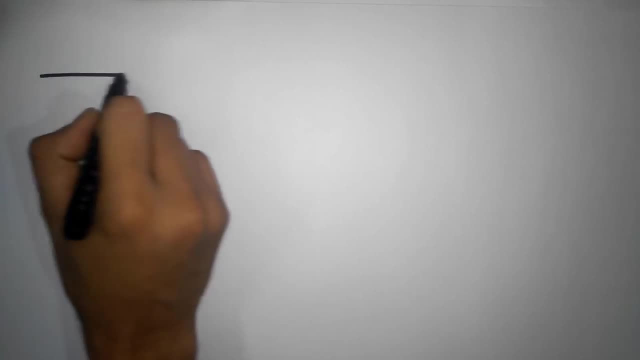 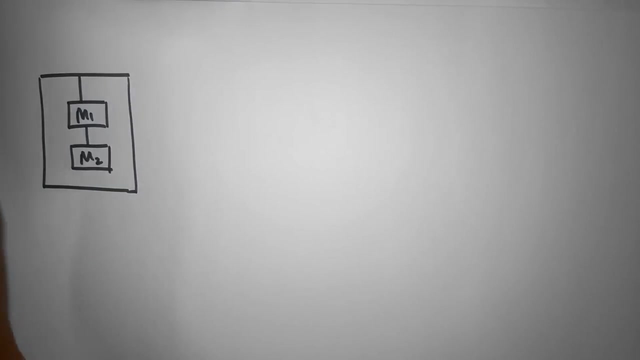 should remain exactly the same. So that's one thing to remember, Alright. So let's take another example. Imagine we are inside an elevator like so And we have two blocks attached to the elevator with the help of a string. Let's call it as m1 and m2.. Okay, and the entire elevator is. 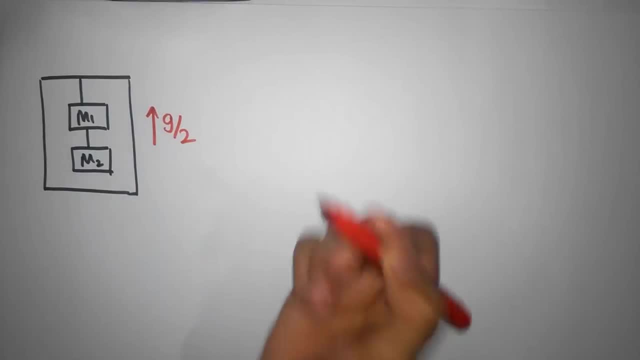 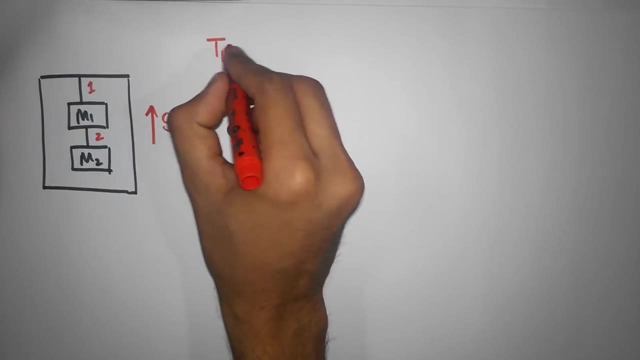 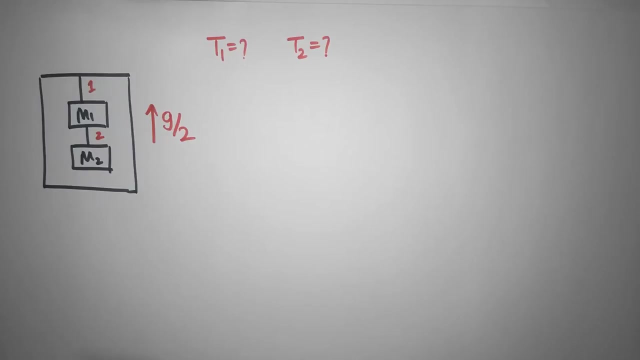 accelerating up, with an acceleration of g by 2.. And the question are: what is the? this is string 1 and this is string 2.. What is the tension in t1?? That's the string 1.. And what is the tension t2 in the string 2?? Okay, now you can do the physics from an inertial. 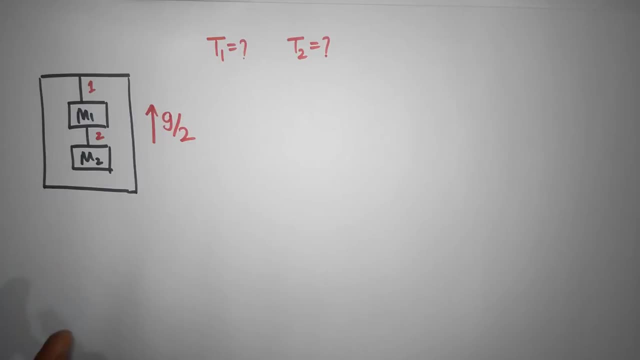 reference frame that is standing outside the elevator or you can do it from inside the elevator. That's non-inertial reference frame. I prefer to do it from the non-inertial reference frame because A I know how to do it, so yeah, But more importantly, from. 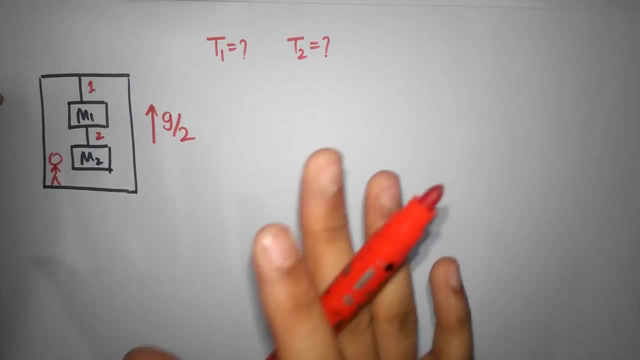 the inertial reference frame. everything is at rest, And I love being at rest because there are no accelerations. the whole thing seems to be in equilibrium. So let's go to the non-inertial reference frame. Let's go to the reference frame. 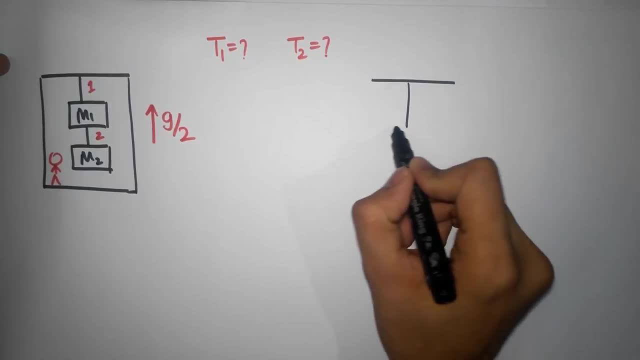 Let's go to the elevator and solve this. So, from that point of view, these guys are just stationary. So there's m1 and there's m2.. Okay, Now let's try and draw all the forces that are going to act on these guys. Clearly there's a force- m2 g- acting over. 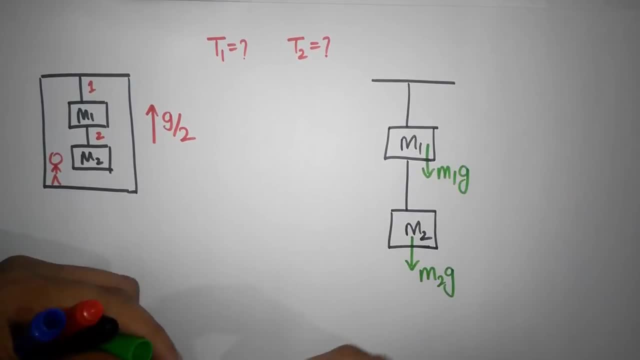 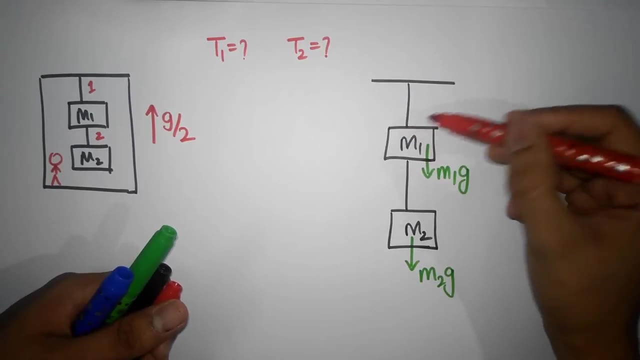 here And on this guy there's m1 g. What other forces? Well, tension, obviously. So what happens here is that this string is going to pull this guy up, just like what we saw before. So this is going to be tension force t1 over here And this string is going to. 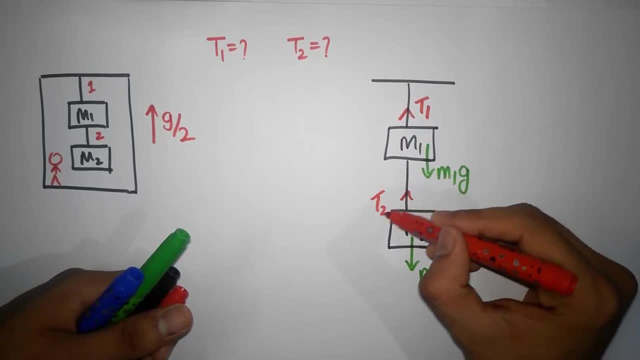 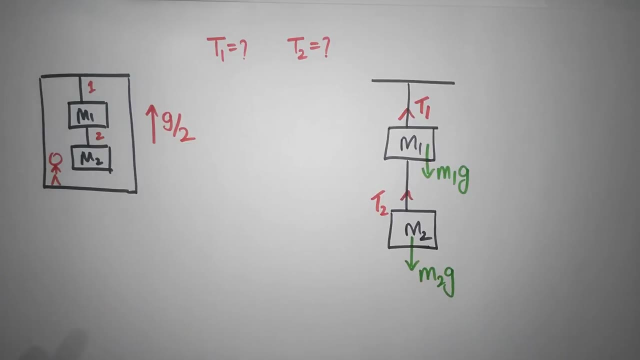 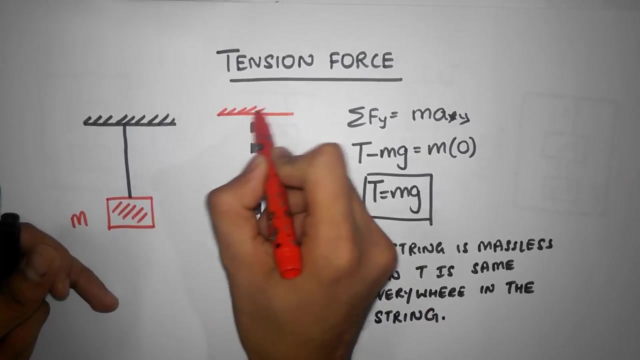 pull this guy up. So there's the tension force t2 here. But notice, the tension force everywhere in the string is exactly the same. Remember what we did last time. And if this was the ceiling, Because the tension force is the same everywhere, even if it's going. 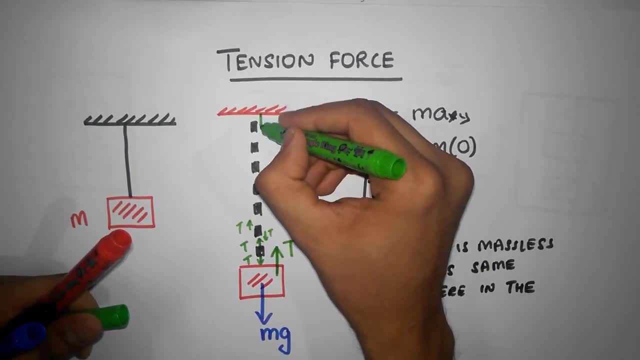 to be the same. even if the tension force is the same everywhere, even if it was the personalities series, that means that there is an energy tension force everywhere. I don't. this particular last part of the string is going to pull on the ceiling down with the. 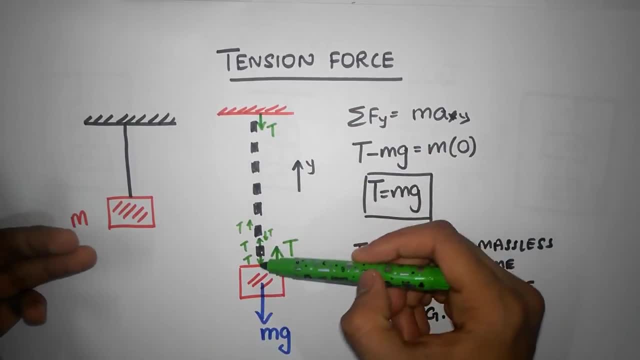 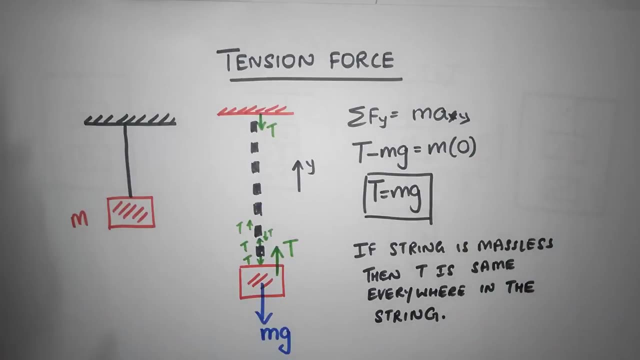 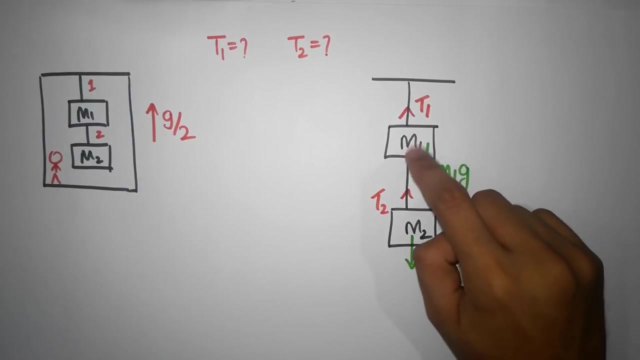 tension force T, and you can pretty much understand this, because you can sort of understand if this was too heavy the ceiling would break, I mean in extreme cases, right. so because of that, even over here the string is going to pull down on this particular block, remember, 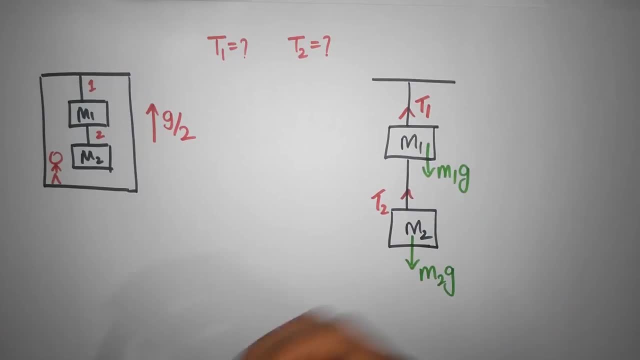 tension force is always a pulling force, so it's going to pull everywhere. so there's a pull down and tension must be the same because it's a massless string. so there's a tension T2 acting over here. so we are now ready to apply equations. oh, I almost forgot this. 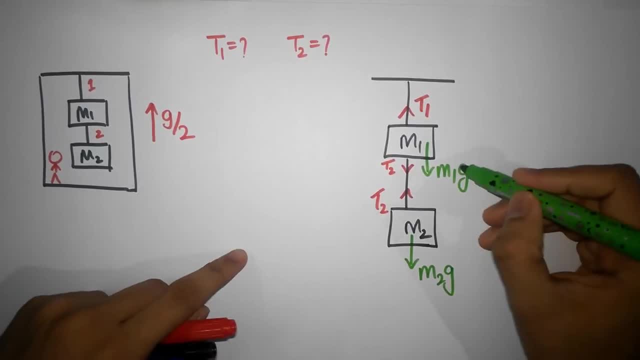 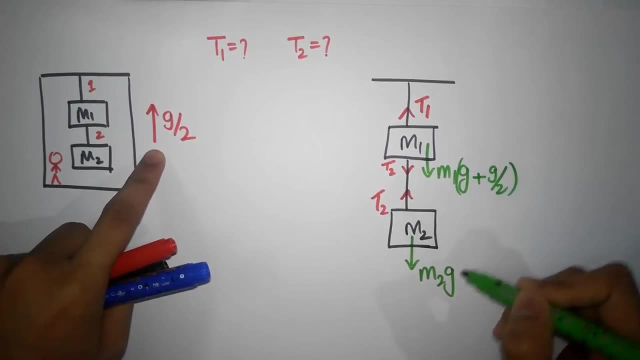 is not G, this is I have to add the fake gravity. how could I ever forget? remember, I have to add fake gravity and that is G by 2. and I'm adding that Because the fake gravity is in the opposite direction. by now, I'm pretty sure you are. 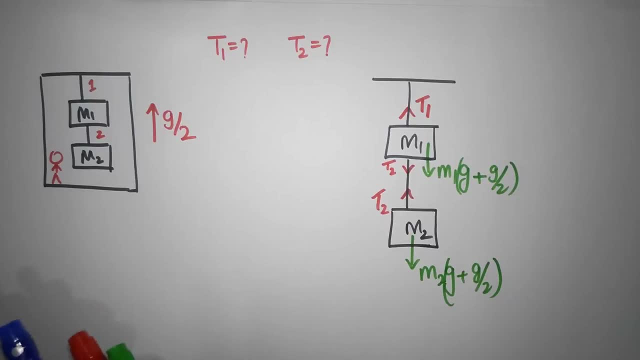 trained with this concept. Okay, let's now apply Newton's second law to both these masses. I'm going to take: upwards is positive. so for mass 1, I will get sigma Fy equal to May, and there are two forces acting and there are three forces acting. there is a tension force acting upwards and there is 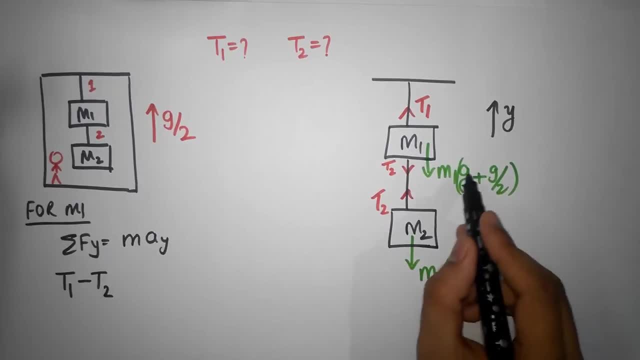 a tension force, T2, acting downwards, and there is a M1, 3G by 2, so there is also downwards. so M1 into 3G divided by 2 should be equal to 0, because from our point of view, there are no accelerations. 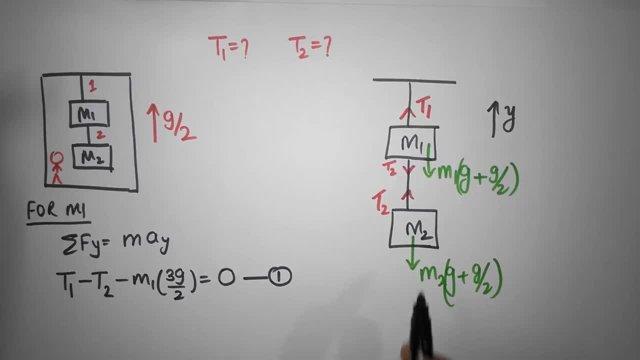 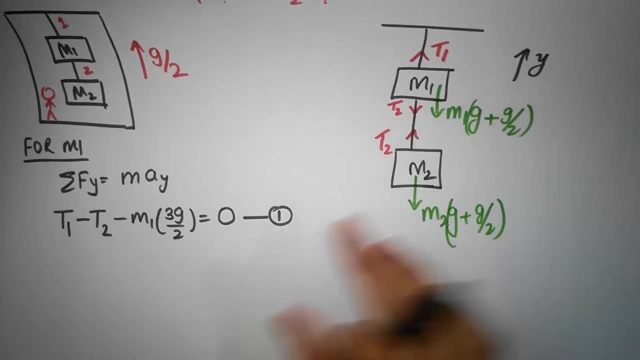 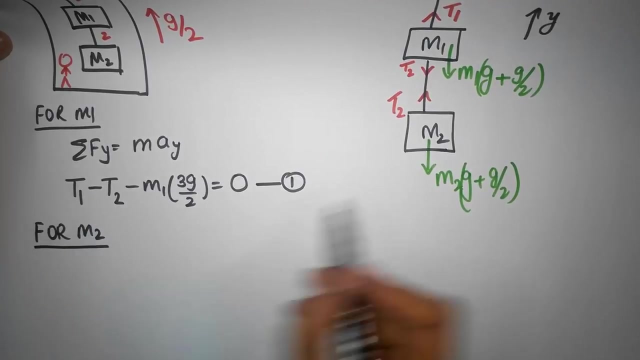 So this is going to be equation number 1 for us. Okay, if I apply this same thing to second block? so let me, okay, so let me apply this to block number 2. and now I would see that there are two forces. one is T2, acting upwards. 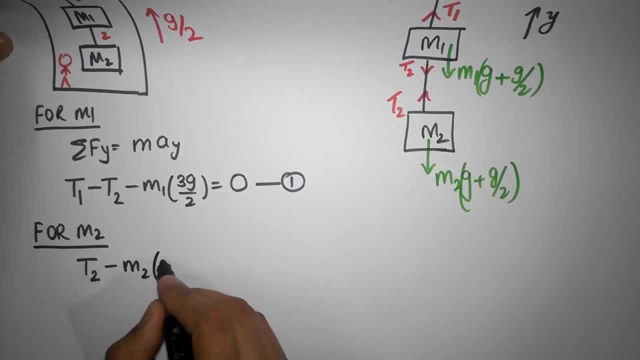 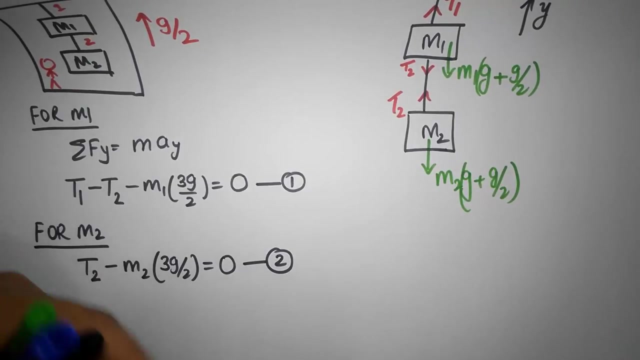 and there is a minus M2 into 3G divided by 2 and that should be equal to 0 again, because no accelerations. So this is equation number 2.. Oh, notice that equation number 2 directly gives me the tension force, so that tension. 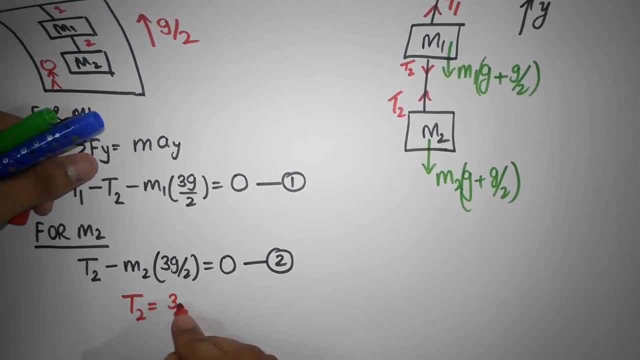 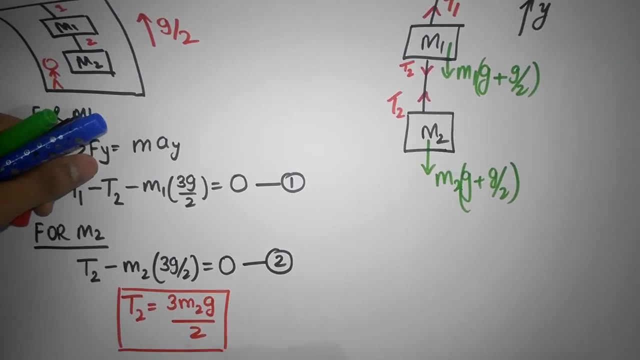 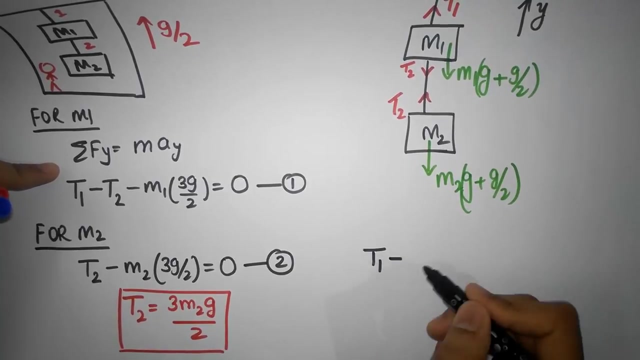 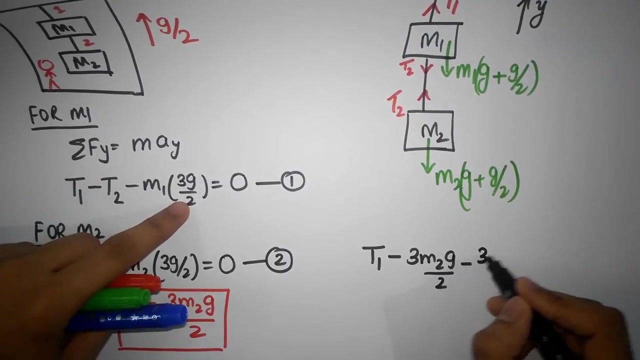 is going to be 3G divided by 2.. Okay, So we got 3M2G divided by 2.. So we got our first answer, and what we'll do now is we'll substitute this guy over here So T1 minus T2, which is 3M2G by 2 minus 3M1G by 2, equal to 0.. 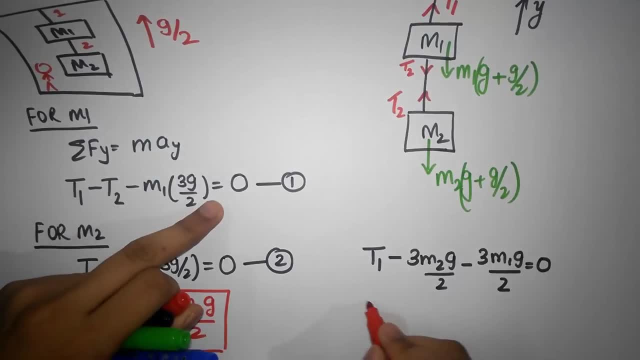 So from this I have my answer. So T1 is: I can take all the common stuff out, I can take 3G by 2 out, and then I get M1 plus M2, tadaa, Now you could have done this actually very fast. you know why? first of all, see it makes. 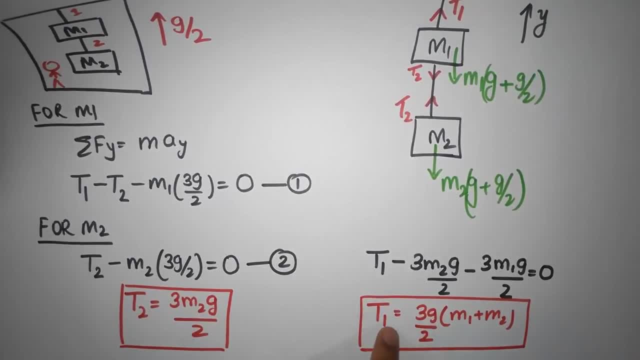 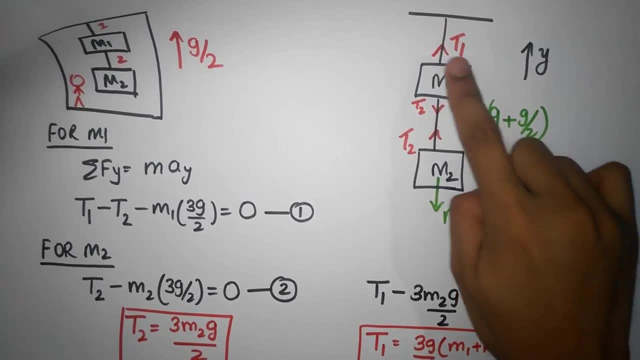 sense that T2 is smaller than T1, in the T1 I have 3G M2 by 2 plus 3G M1 by 2, that makes sense right, because this string not only has to support the weight of this guy, but he also. 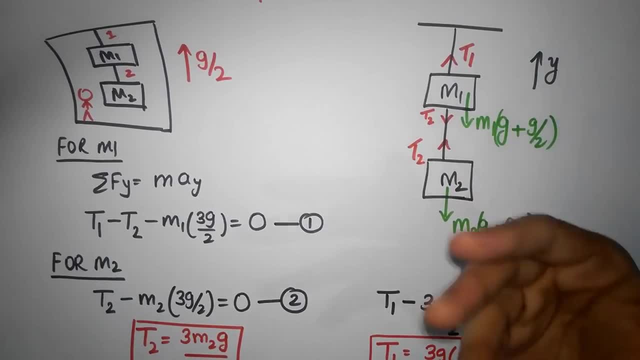 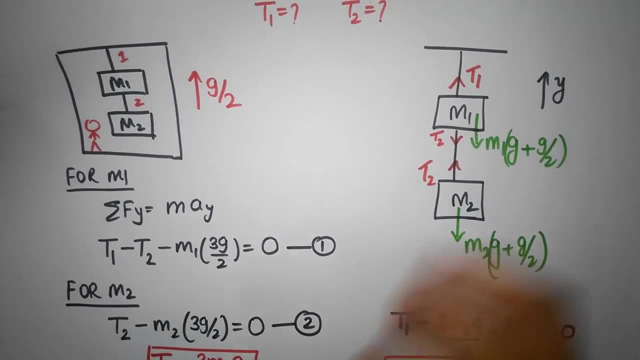 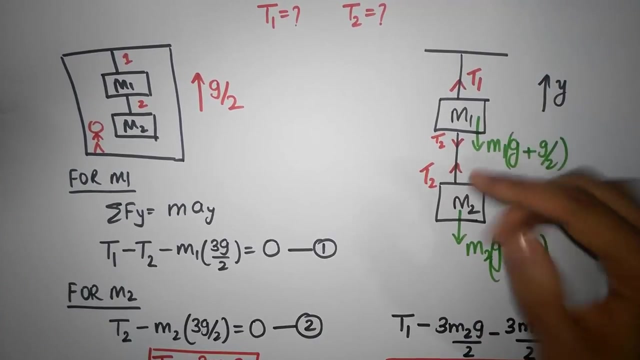 has to support the weight of that guy, or at least in our- what do we say? in our traditional language or our trivial language, we would say that. But as long as physics is concerned, don't think that this string is bearing the weight of M1 and M2, instead, it's much. it's much better and you know, it's more accurate to.